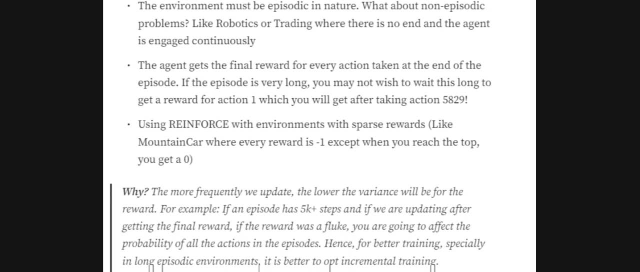 the episode to end to get to the final reward that we can get. Reinforced algorithm may be problematic for sparse reward systems as well, So last time I tried my mountain car training environment from OpenAI gym using reinforced algorithm, It was very hard to train. 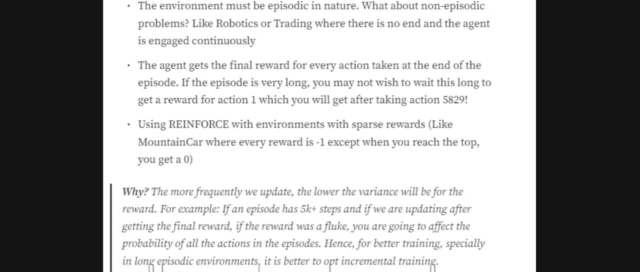 because the final reward that comes is the only reward that you are getting. else, all the rewards are minus one. So reinforced algorithm is not that great with sparse reward systems as well. Now to a point where we are saying that when the episode is long, we are getting a reward in. 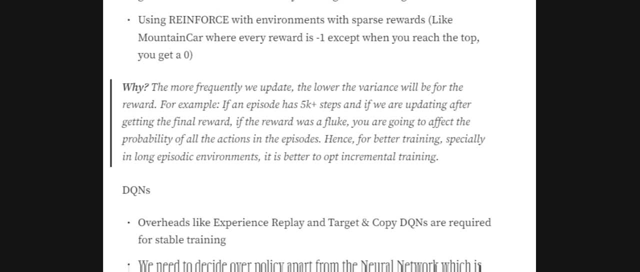 the end of the episode. Why it is problematic? because the more frequently we update the system, the lower the variance will be. For example, if I episode has 5000 steps and we are updating after getting the final reward and assume that the final reward is a fluke, So by chance you get some high or low reward. So in that case that would be. 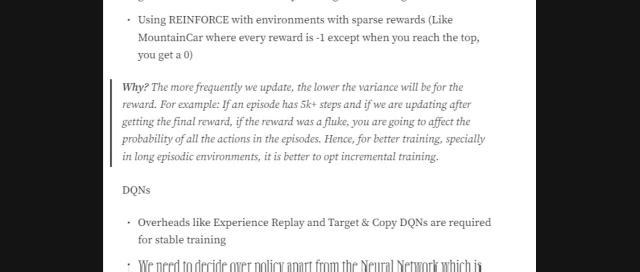 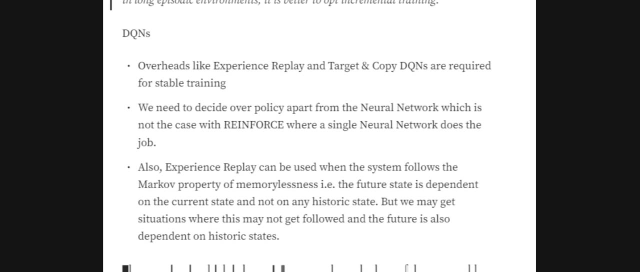 good, that would get updated throughout the system. So we would wish to update it more frequently, as we do in DQNs. So in a previous video I have already also explained how to use DQNs, So let's understand a few problems with DQNs as well. So, already explained in that video, we would be using 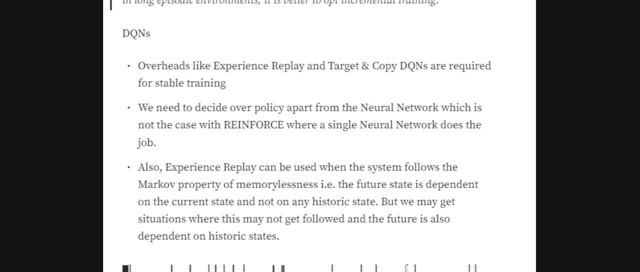 overheads such as experience, replay, target and copy DQNs to make the training stable. Now, this is always an overhead. we need to code a lot of things. apart from it is time consuming as well. Apart from that, we also need to decide over 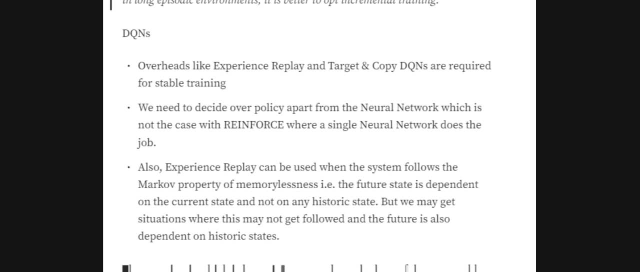 the policy to be taken, as DQNs are majorly belonging to value-based methods, where we are predicting the Q value for an action and not directly the probability for the action In a combination of the Q value. alongside the policy that we choose, we would be finally taking. 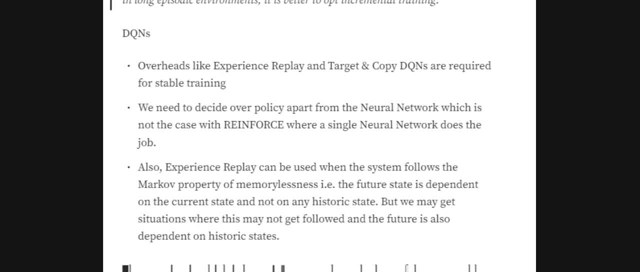 an action which is not in line with reinforced. So in reinforced we are not having any such sort of overheads. Apart from that, experience replay that we use to stabilize the training is based on the idea of Markov property of memorylessness. That means that the future state is dependent on the 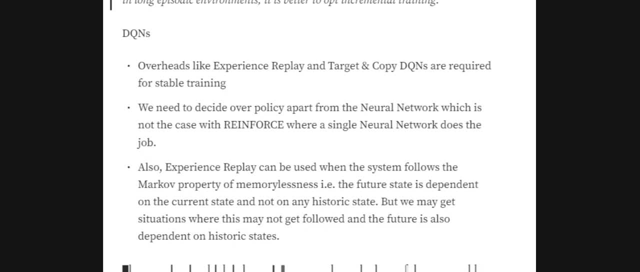 current state. But we might have such systems where the future state may depend on multiple previous states, right? So in that case experience replay might not be of great help and training DQNs would be tough. So here we have seen that there are two major like some problems with both. 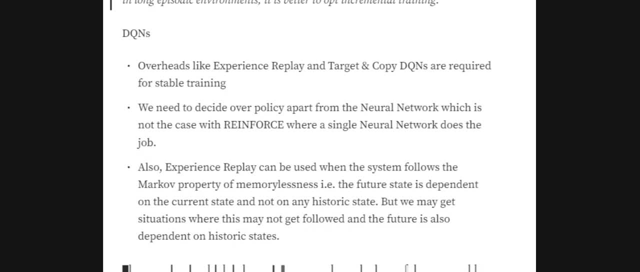 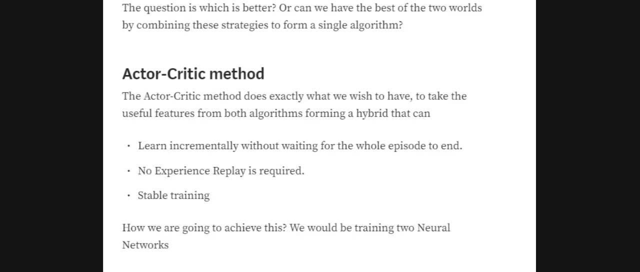 value-based methods as well as policy networks. Policy network was a reinforced algorithm and value-based method was DQNs. Now can we combine these two models to overcome all these problems and get the best of the two worlds? Yes, So we will be discussing about the actor. 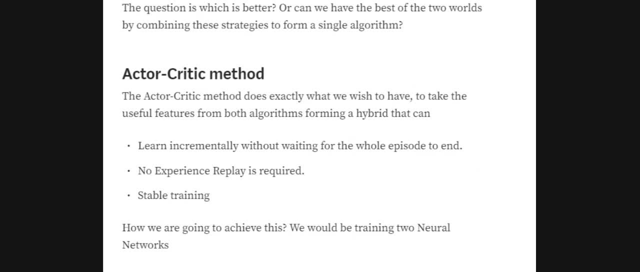 critic method today, which is sort of a hybrid model that is coming out of DQNs plus reinforced algorithm. So, basically, the things that we are getting in case of our actor critic method is that we are not waiting for the whole episode to end. There is no experience, replay used and training is. 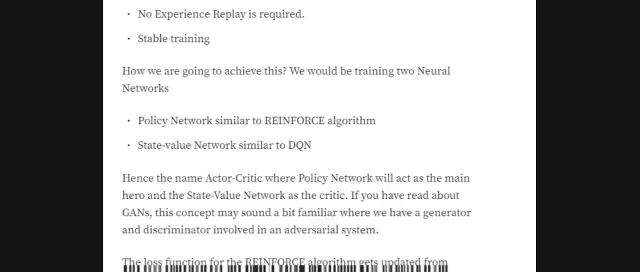 also stable. So how do we achieve that? So in actor critic, as the name is suggesting, we would be using two neural networks: One is actor and other is a critique. So the actor would be the policy network which we use in case of reinforced algorithm, and the critique would be the state value network. 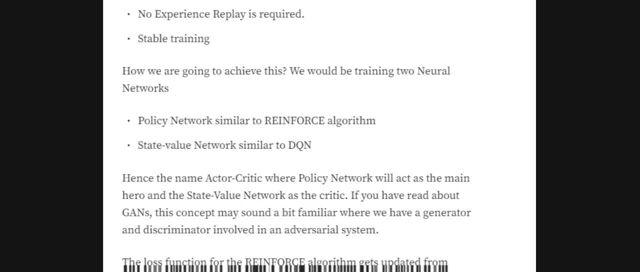 that which is very similar to DQNs. So you got my point. So we have combined these two models together and now we are calling the action. So we are calling the action, and we are calling the action. So we are calling it as actor critique, where the major algorithm would be policy network and its 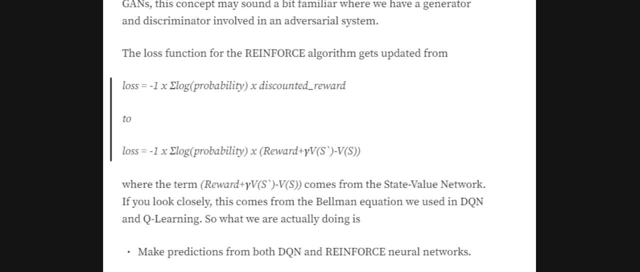 critique would be state value network that is a DQN. So the loss function that we used to update in reinforced algorithm was minus one into summation of log probability into discounted rewards. But now in case of actor critic method, the loss function for the policy network would 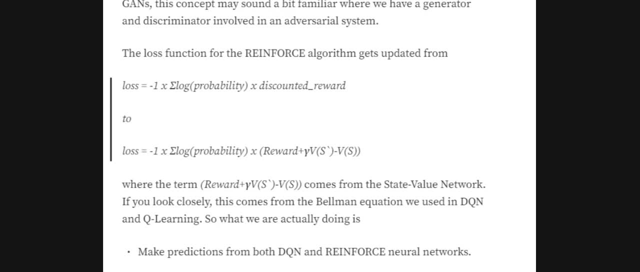 become minus one into summation of log probability, into reward plus gamma value function for the Q value for the future state minus Q value for the current state. So we are calling it as actor critique state. So here you can see that this particular extra term discounted reward we have removed and 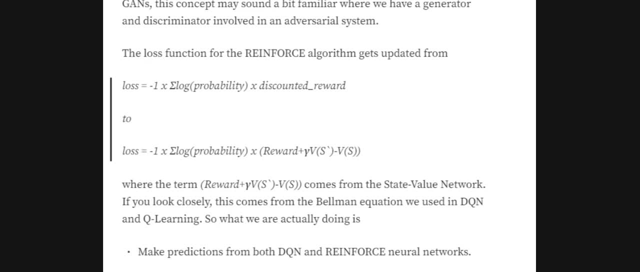 this extra term that we are getting, we would be getting from the DQN that we are training. that is the critique, As you can see, that the Q values for the future state and the current state would be given by the DQN, And there is a term very similar that we have already discussed in the 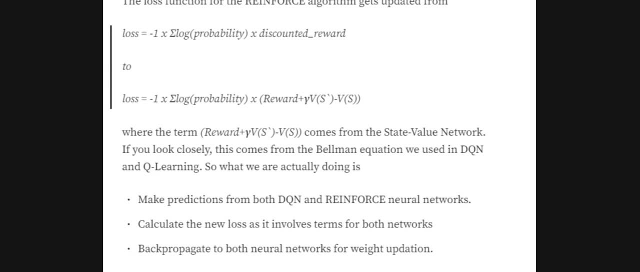 Bellman equation. So it is very similar on those lines. only Now we would also be having a loss function for the DQN also, but that is very similar, which is a mean square error for target Q value and predicted Q value. So the total loss function for the whole algorithm actor critic method would be: 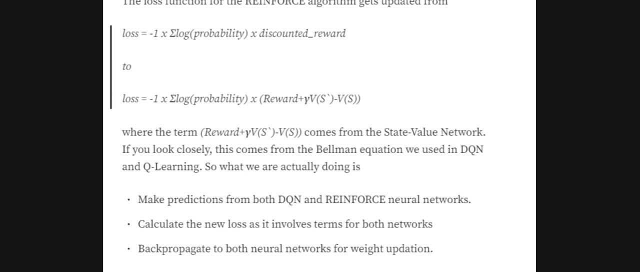 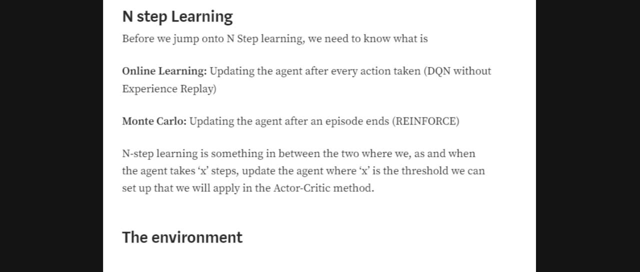 this particular loss plus the mean square error between target Q value and predicted Q value. There would be one more concept that I need to introduce before jumping in. that is called as an end step learning. So basically, there are three types of learning that we can do in reinforcement. 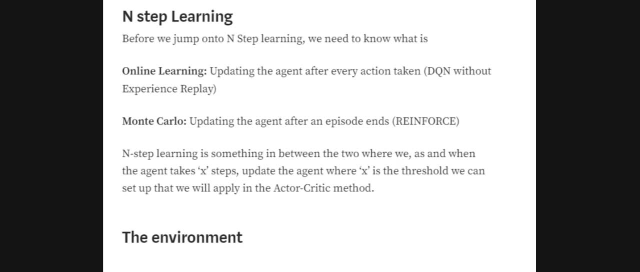 learning. One is online learning. that is, we are updating the agent after every step that we that we would have done in case of DQNs if we wouldn't have been using experience replay. So, if you remember, experience replay was more of a buffer We were. 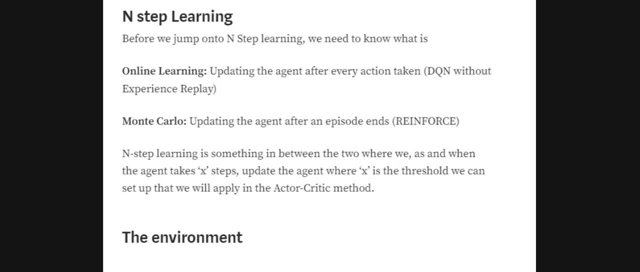 sharing some samples and then eventually updating the whole model. If we won't be using experience replay, then, case of DQNs, you would be updating it after every action taken. that is called as online learning and Monte Carlo. So Monte Carlo I have already discussed. So, in case of Monte Carlo, we 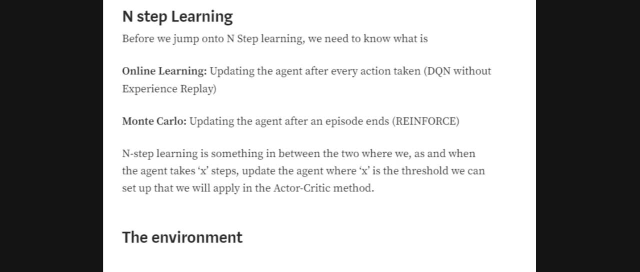 wait for the whole episode to end and then update the values, which was the case of reinforced algorithm. Now, end step learning is somewhere in between these two learnings. So what we would be doing is that we would be waiting for some x steps to be taken. 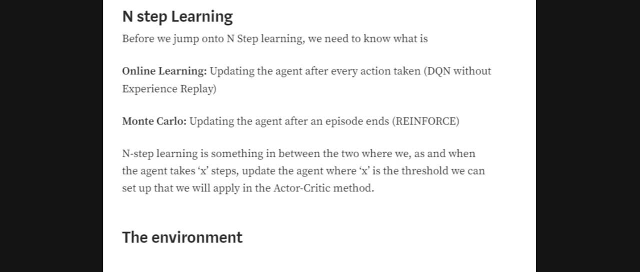 So what we would be doing is that we would be waiting for some x steps to be taken. We won't wait for the algorithm for the episode to end, but we will wait till some end steps and eventually, once the end steps happen, we will be training the whole system. 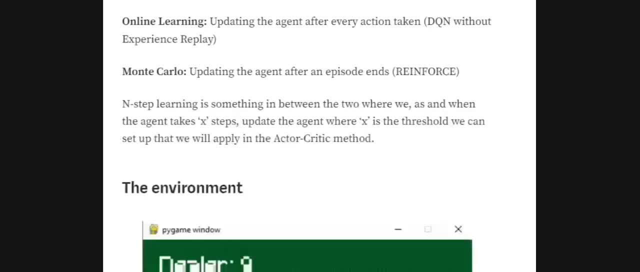 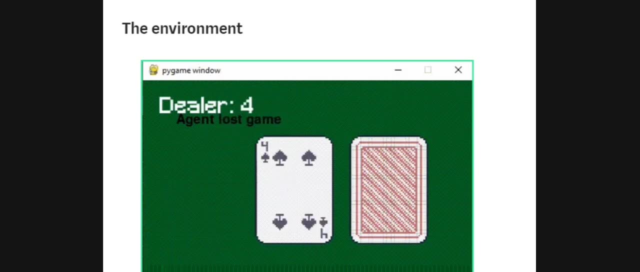 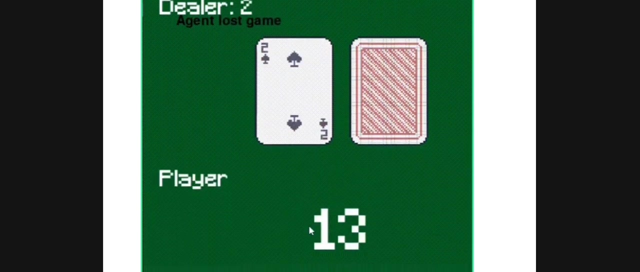 so that we can maintain, we can update the system more frequently. So the environment that we will be training now would be blackjack, So I'm testing out with different environments every time. This time it is a card game that is coming from OpenAI Gym, So here you can see that the how the UI looks like. So I will tell you what are the rules for. 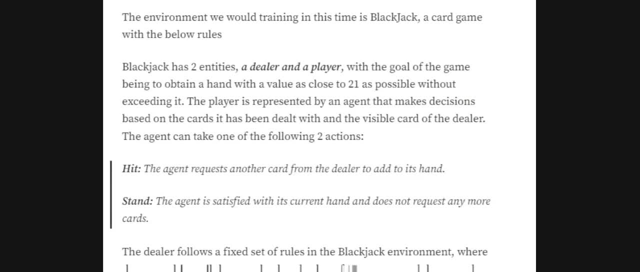 blackjack. So in black, in case of blackjack, we have two major players. one is a dealer, another is a player, so the player would be our agent. Now, the goal of the game is that to obtain a hand of cards which has a value close to 21. it should not cross 21, right, it should be close to 21.. The agent can. 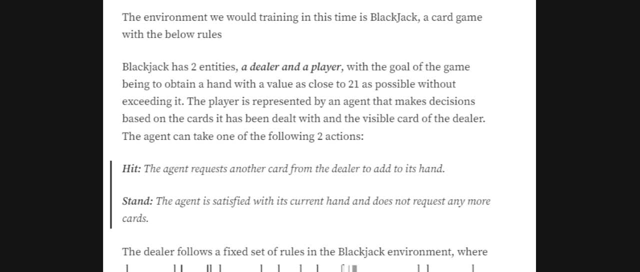 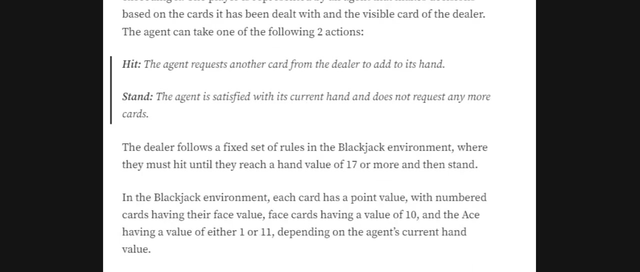 take two actions at a time. to out one action out of the two possible action at a time, hit the agent. request for another card from the deck stand. the agent is satisfied with his current hand and does not require any more cards. So there are two actions that are possible in this game. Apart from that, the dealer follows a fixed 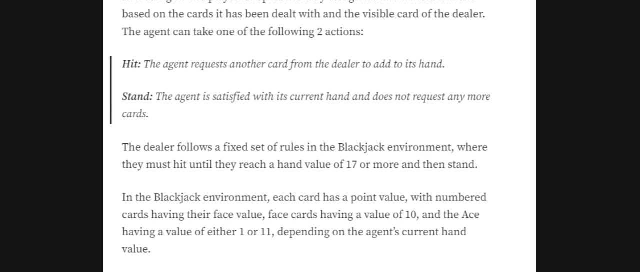 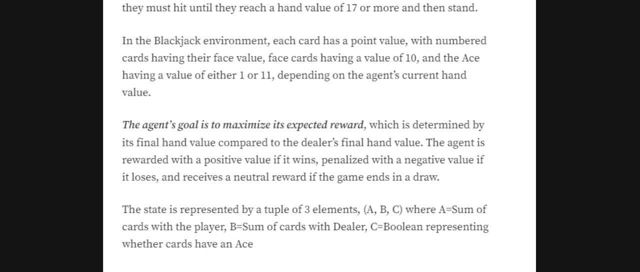 set of rules in OpenAI Gym environment where he would be hitting again and again until his value reaches 17 or more and then stand. So in the blackjack environment, each card has a point value. so like: if the card is two, the point value is two, if the card is three, the point value is three. 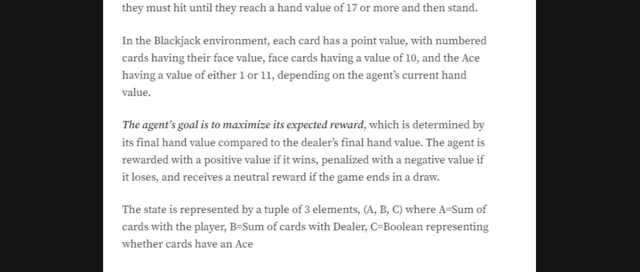 and so on. So for the face cards like jack king queen, it is 10 and for the ace it can be one or 11, depending upon the current combination. you wish to choose it how you're considering it. So, for example, if you have a hand with ace and nine and two, the total value can be either taken. 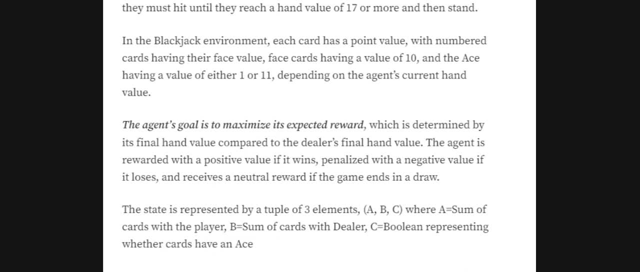 as 12, because nine plus two is 11 and ace is equals to one, then can be 12, or it can be 11 plus 9 plus 2, that is 22.. So, depending upon how you are playing or depending upon a strategy, you can change the value for the ace. 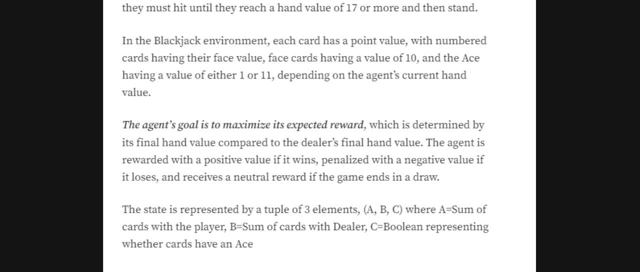 it is interchangeable. Now, the goal of the game is to maximize the expected reward. so, uh, the case is that the agent will win the game when, uh his uh, the value of the uh cards in his hand is more than the dealer's card value of the dealer's card and less than 21.. The state is 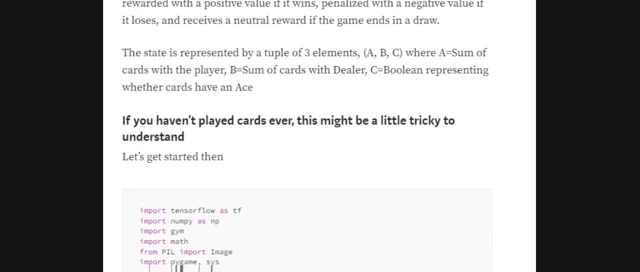 represented by a tuple of three elements in OpenAI Gym, where a- uh, with, as you can see, a tuple a, comma b, where a is the sum of card with the player, b is the sum of cards of the dealer and c is the boolean representing whether the, whether the player's card has an ace or not, because ace is. 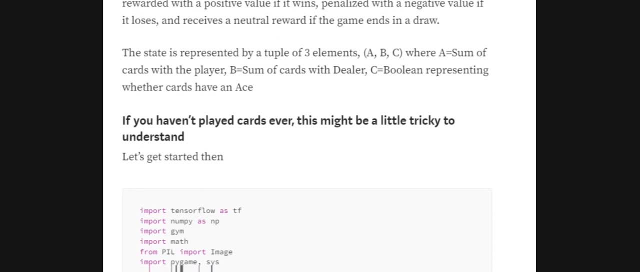 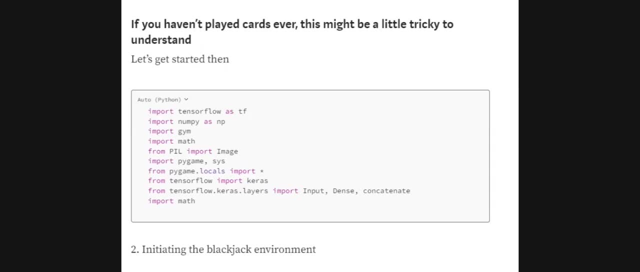 interchangeable right. so, depending upon that, this is the state space that we get from OpenAI Gym for blackjack. uh, we will be discussing about the codes for coding out a actor critique method in reinforcement learning to train blackjack environment in OpenAI Gym. So let's get started. so, first of all, we will be importing all the required libraries. 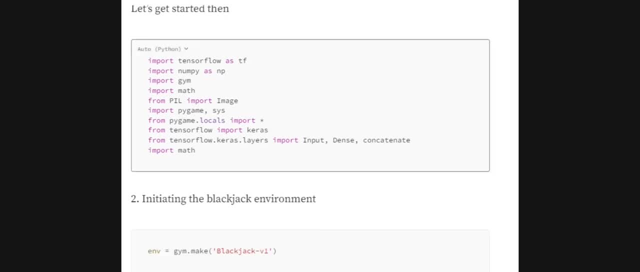 So let's get started. so, first of all, we will be importing all the required libraries. So let's get started. so, first of all, we will be importing all the required libraries. So you can see that i've also imported pygame. pygame would be helping us to visualize the whole. 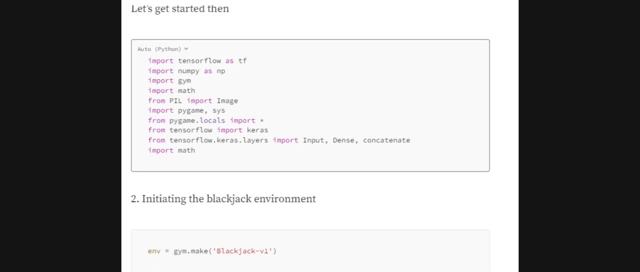 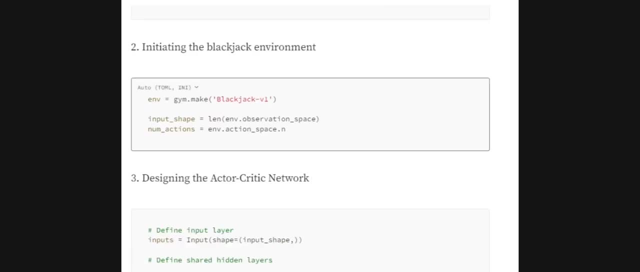 uh environment. uh, in our local system. apart from that, i've also put tensorflow so that i can train the whole neural network into tensorflow. next i would be initiating the blackjack environment i. this is something that we have already seen- a previous video, how we initiate OpenAI Gym. 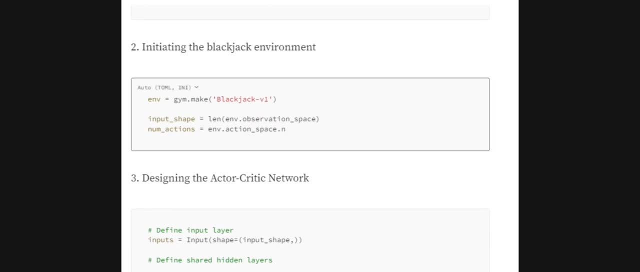 environments and we are taking the input shape, that is, input shape is basically the shape of the state space that we're having. that would be, uh, that would be three year, because, uh, uh, in blackjack, the, the dimension of a state variable is three and number of actions, basically. 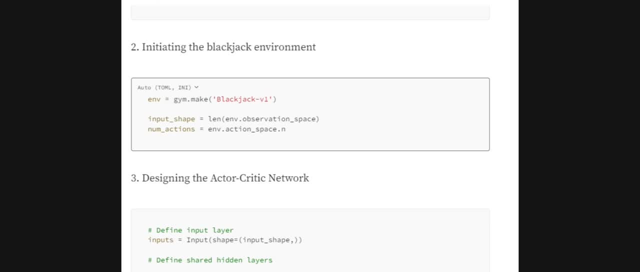 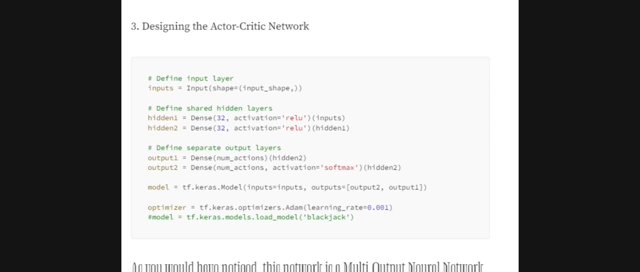 the total number of actions that the agent can take. that is equals to two. in case of blackjack, that is hit or stand. now we will be designing the actor critique network, so i would be using a multi-output network for designing this actor critic network. so what is a multi-output network? 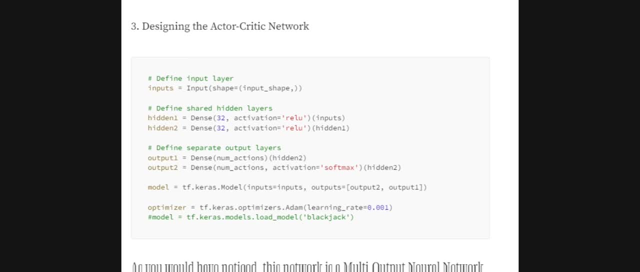 so in case of multi-output network, we have the same input, the whole body remains the same, but the but the model is able to give multiple outputs of from diff, of different ranges. so here you can see that, uh, i have first of all taken an input, then i've designed the inner, the hidden layers of the network. now, here you can. 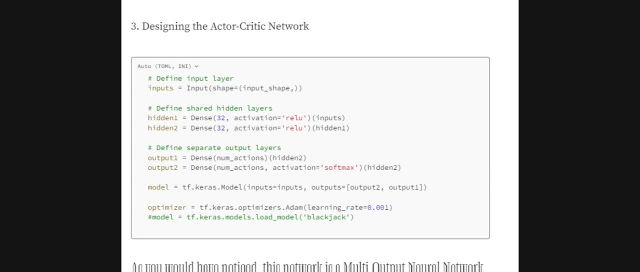 see that they are having two outputs now. one output is directly dense layer, without any activation, and another output is the activation level, softmax. so the other layer is basically probabilities and second is basically the q values that we would be getting for uh that we are, that we would be getting for the critique, and softmax represents uh, the 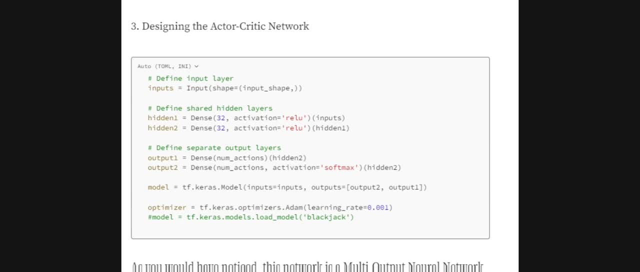 probability for the actions that the actor will be generating. so output one is the head for the critique and output is the head for the actor. now here you can see that how i am compiling the model. so inputs remain input, but the output is a list of two values: output to an output one and eventually, 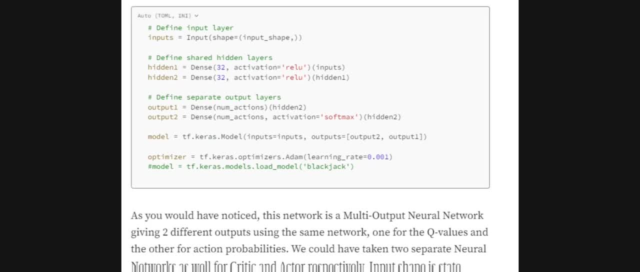 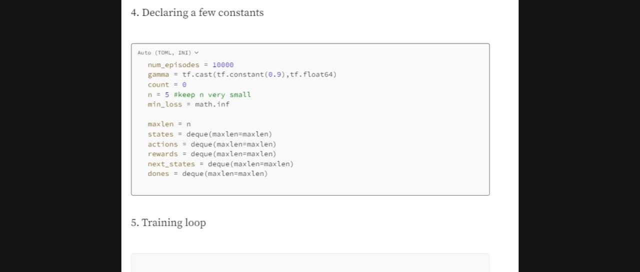 the optimizer is just, uh, one optimizer. that would be helping us to optimize the whole network. you can also design two different networks, that is up to your wish. i will be declaring a few constants here: the total number of episodes for which i wish to train the co? uh, train the model. 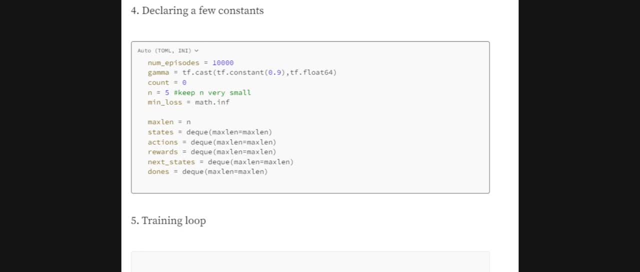 the gamma value that i would be using in updating in the loss function, um, and equals to five for the end step, learning. so after every five step we will be updating the environment and state action reward. next steps are done are basically list that we wish to store the values in. 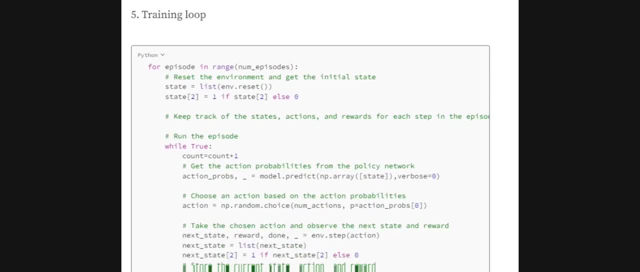 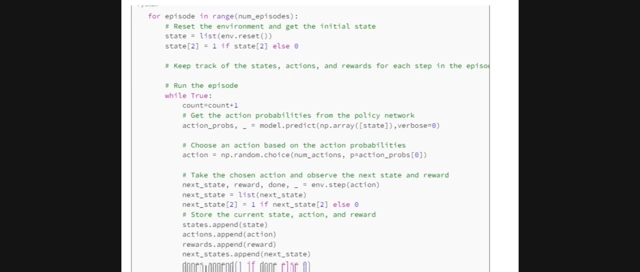 uh, now coming to the training loop, so it is the most important thing. so, first of all, uh, we will be looping over the total number of episodes for which we used to train and then resetting the environment, and for every episode that we had, uh, For every episode that we are training the agent for, we would be first inputting the 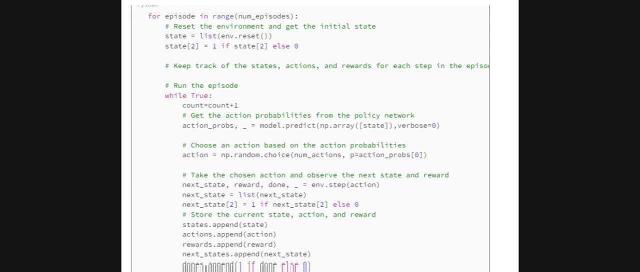 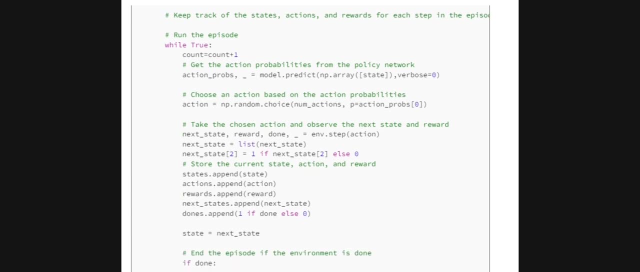 state and take the action probabilities, we are skipping the Q values. As you know that we have taken a multi-output network, so it would be giving us two outputs, So we are ignoring the second output here you can see, Now, depending upon the probabilities, we are taking an action and then we are getting the 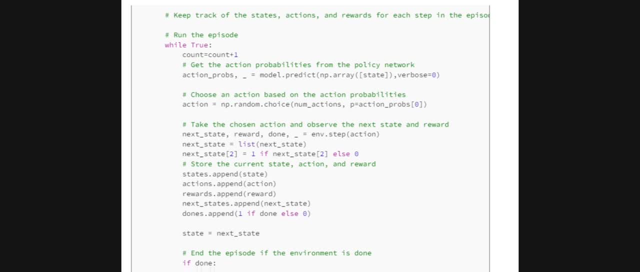 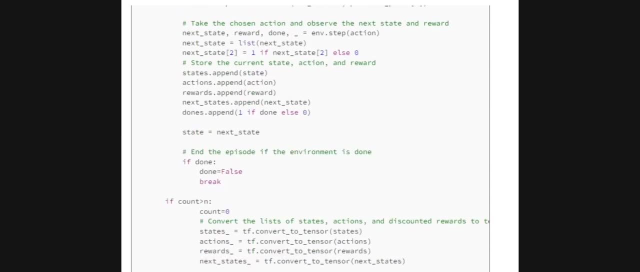 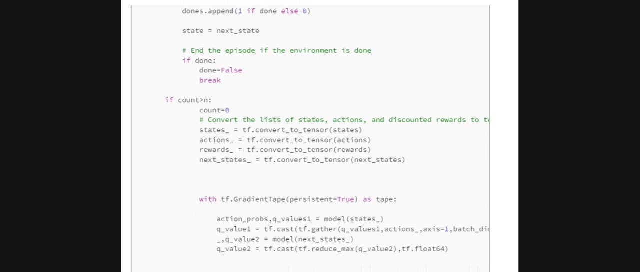 next state, the reward, the done flag, by inputting that action to the environment and then storing all these values in the DQs that we have mentioned, that we have initialized earlier. Now, here you can see that here the main crux is, once the count is greater than n, that 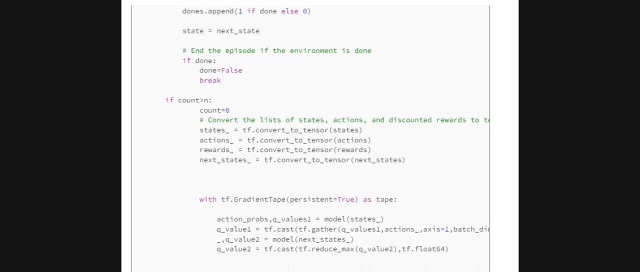 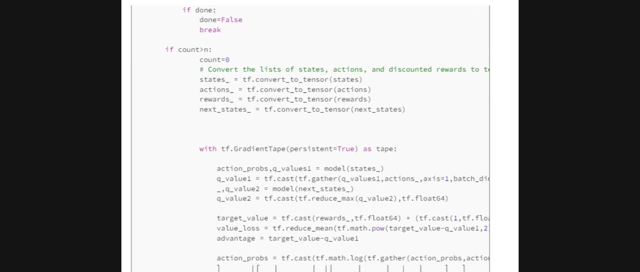 is the number of steps that we have. we are resetting. the count equals to zero, So it is basically after every five steps. we wish to update the model. We are converting all the DQs that we have into tensors and then using gradient tape. 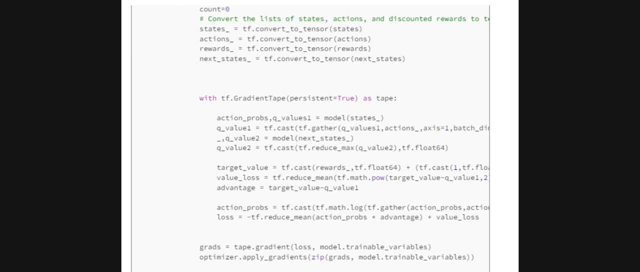 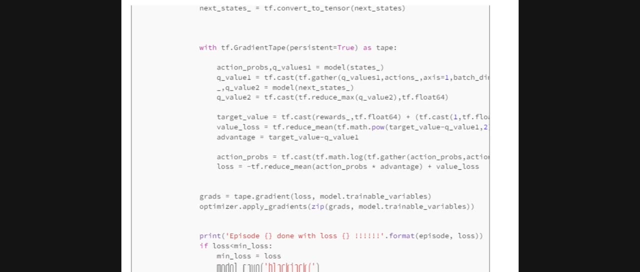 I would be first calculating the loss functions and then applying those gradients. So here you can see how the loss function is calculated. So we are getting probabilities for the action And the Q values for the actions. Using the model, we are recalculating them. 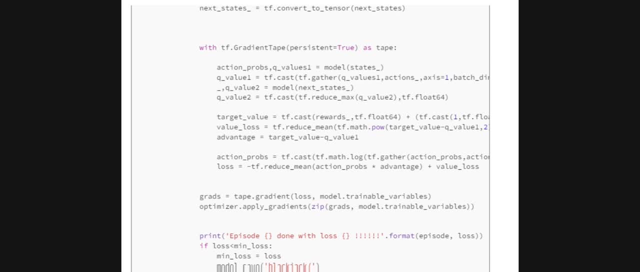 Using tfgether as Q values would be for all the possible actions. we would be getting the Q value for the specific action that we have taken. Now we would be again using the model to calculate the Q value for the next state. As you saw in the loss functions that I mentioned earlier, we are using the Q value for the. 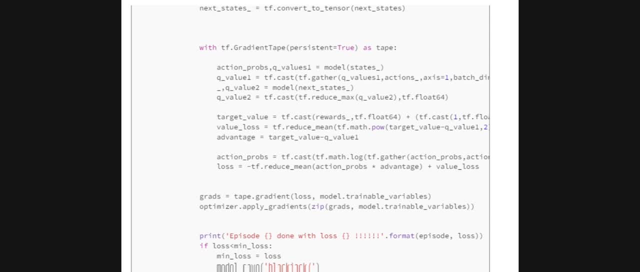 future state as well as the current state. So here we are ignoring the action probabilities and just taking the Q value for the next state And then again taking the maximum value out of that Q value too. That is, we are considering the maximum value from the next state Q value. 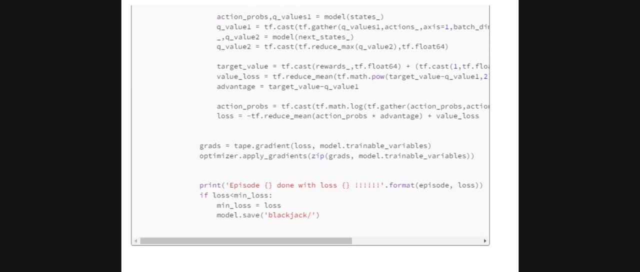 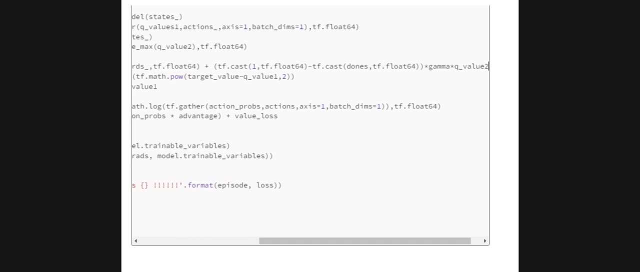 Now we are calculating the target value that we would be considering for training our critique network. So it is nothing but reward plus gamma into Q value too. That is the reward that we got into the gamma, into the future state. So here we are calculating the target value that we would be considering for training. 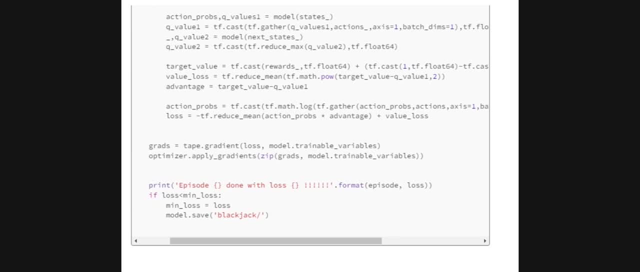 our critique network. So we would be considering the future reward that we would have got. So target value becomes this for the critique. So we are calculating the value loss term. So, as I told you, we would be having two losses: One is the policy network loss and the other is the value loss. 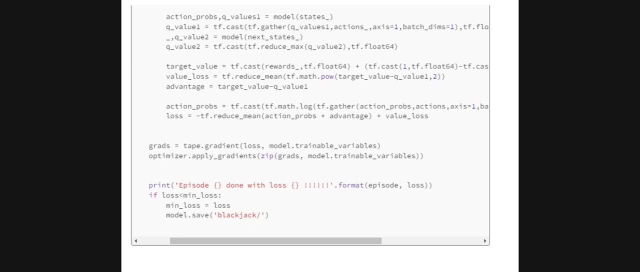 So the value loss is equal to target value minus the current Q value whole square and taking a mean over it. So its very mean squared error that we call. that is what is getting implemented here. For this we are calculating a term called advantage. 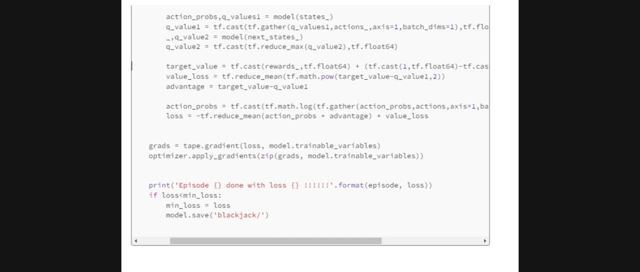 So, as I told you in the beginning that we would be calling this as advantage on some cases, actor 2 critique method. so here is the advantage that we're calculating. so advantage is nothing but target value minus q value. and then we're again. we are getting the action probabilities. 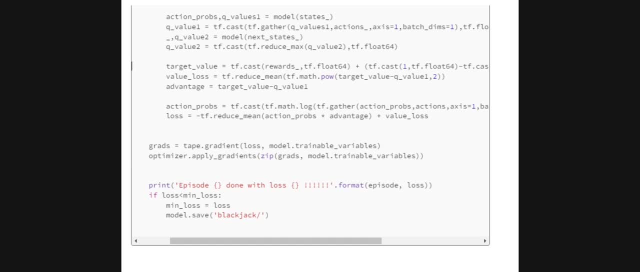 for the action that we have taken. uh, as this would again action the for the first line that, as you can see, gives us the output for our probabilities for all the actions. so we need to get the probability for the specific action that we have taken and then calculate the final. 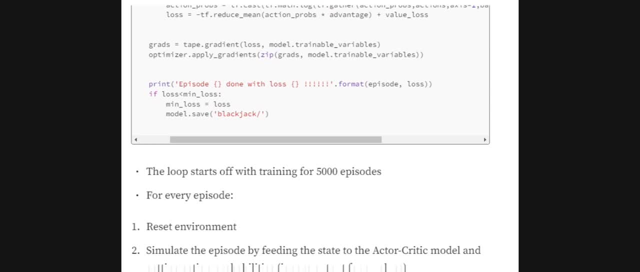 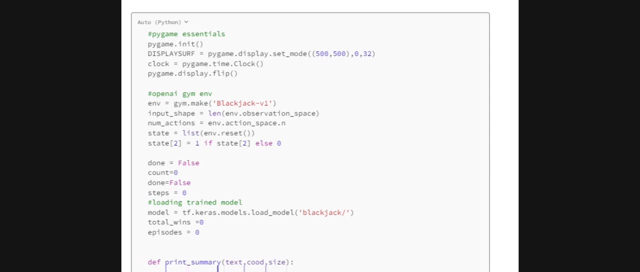 loss, as mentioned earlier, and then applying gradient tape. now this particular code snippet i would be using to visualize the whole network, as i have showed you earlier a gif in the blog itself. so this code will help us to visualize this. i have already explained this whole code snippet. 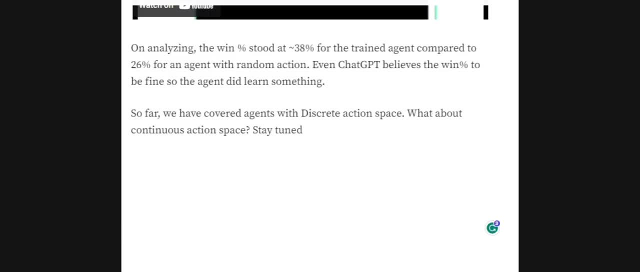 in one of my previous videos so you can go and visit it. so on, uh, analyzing the winner percentage for the trained agent stood for 38 percent of the total episodes, uh, that we have. so i played thousand games, out of which i- we were that agent- was able to win nearly 38 percent of. 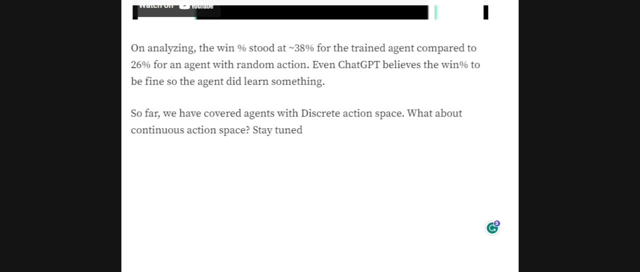 of the total games. now i again played the same game with a random agent and the success rate was about 26. so here you can see that we have got an increase of 12 after training the agent. i firmly believe that. okay, uh, if we would have trained for some longer time. 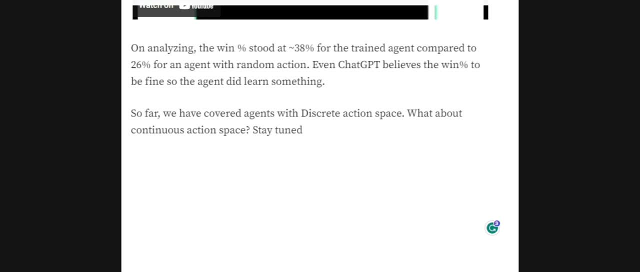 the result would have been great, but still, uh, here you can see that a direct impact where the agent is able to now play blackjack, uh, comparatively better than a random player.